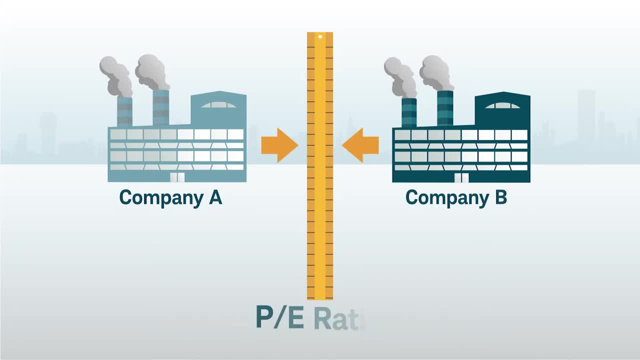 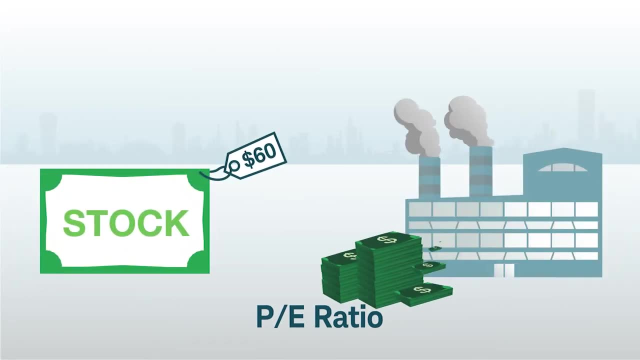 we need a common measurement, such as the price-to-earnings or P-E ratio. The P-E ratio simply compares a stock's price to its company earnings or profit. Now back to our video. For example, let's say Company A is located in Wisconsin, which gets a lot of snow. Therefore, 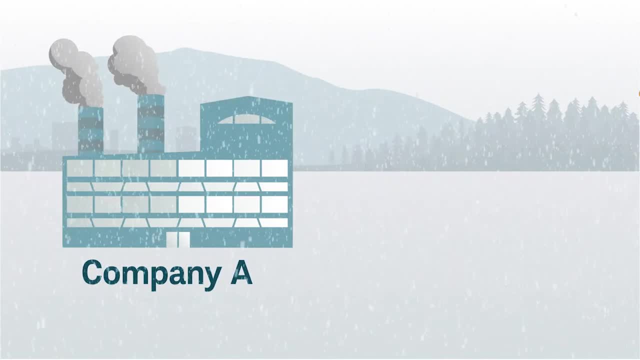 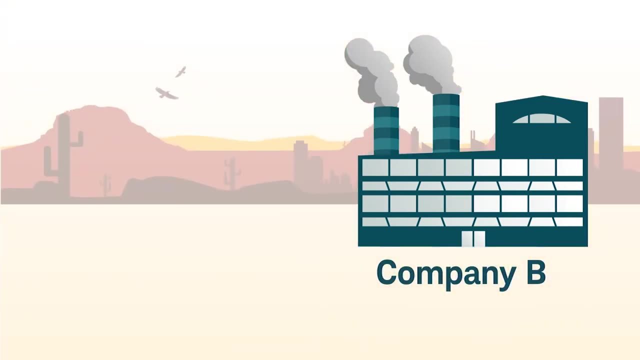 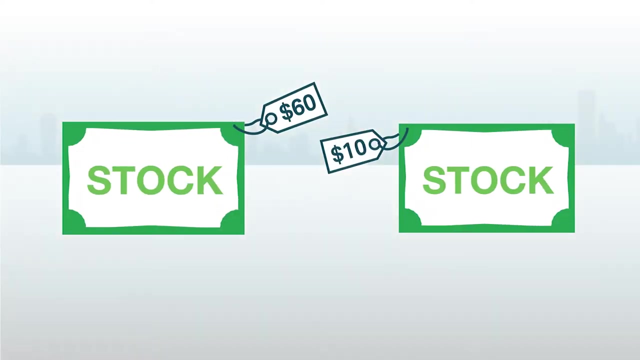 Company A sells a lot of shovels and earns a profit of $100,000 a year. Company B is located in Texas. While Texas is a big state with a high population, it doesn't receive much snow. Therefore, Company B only earns a profit of $10,000 a year. We know each stock's share price. 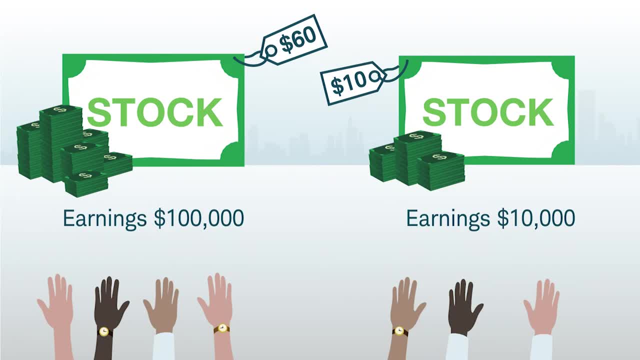 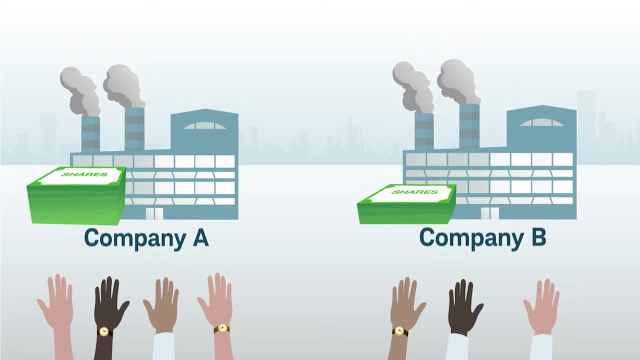 and each company's earnings, but we don't know how many shares have claim on the earnings. To put it another way, we need to know how many shares the company has issued to calculate the value of each share relative to the company's overall earnings. This calculation is known as 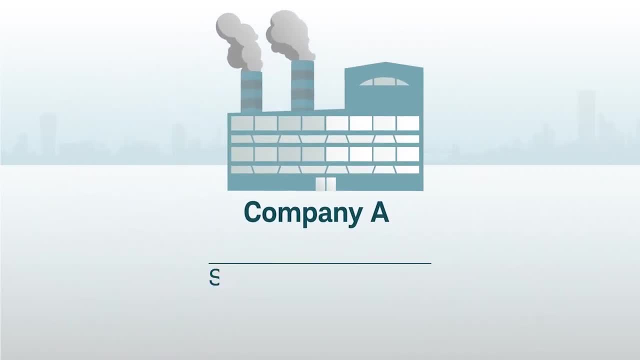 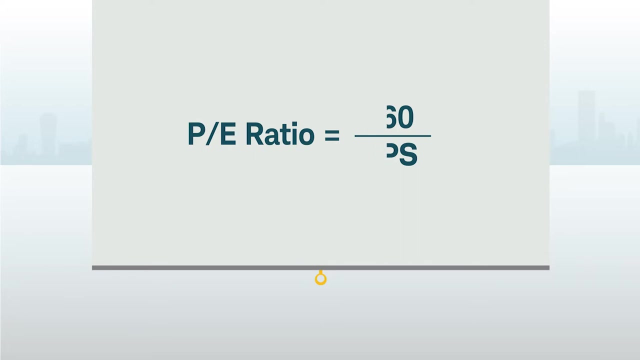 earnings per share or EPS. Because Company A has 50,000 outstanding shares and $100,000 in earnings, each share has a claim on an EPS of $2.. Now that we have Company A's EPS, we can calculate the P-E ratio At a price of $60 per share and an EPS of $2,. 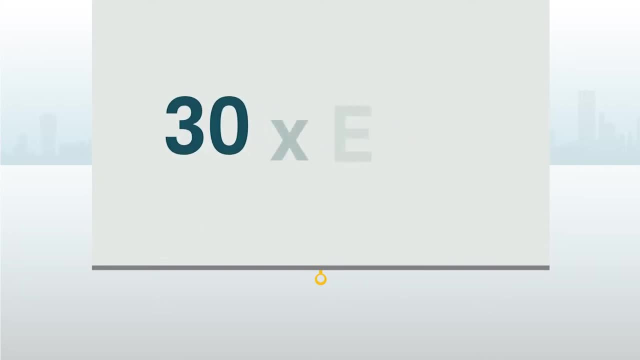 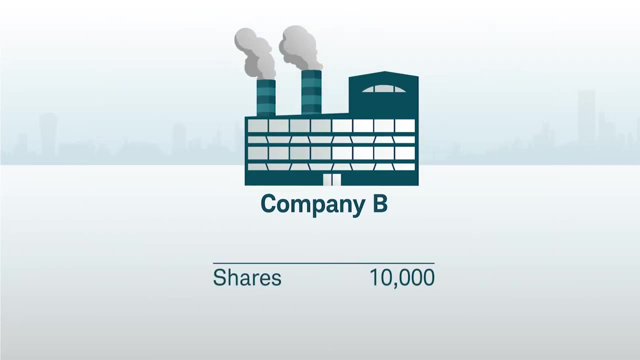 Company A's P-E ratio is 30. This means its stock is trading at 30 times its earnings per share. Let's calculate Company B's P-E ratio. It has 10,000 outstanding shares and $10,000 in earnings. 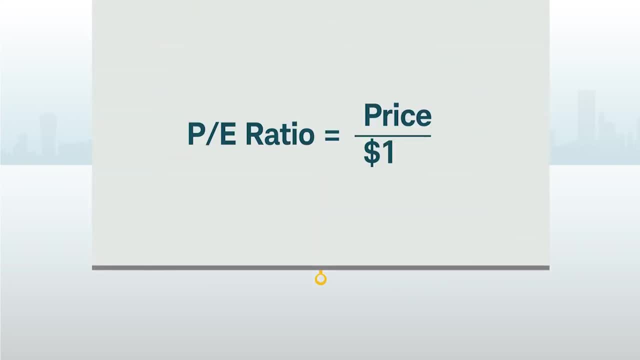 resulting in an EPS of $1.. The stock is at $10 per share, which means Company B is trading at 10 times its earnings or has a P-E ratio of 10.. In this example, Company B may be a better value. 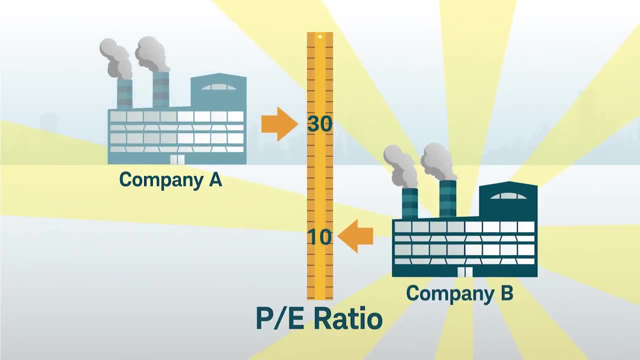 not because it has a lower stock price, but because it has a lower P-E ratio. In other words, the lower the P-E, the less an investor is paying per dollar of a company's overall earnings. Although the P-E ratio is the most common valuation measurement, it isn't the only. 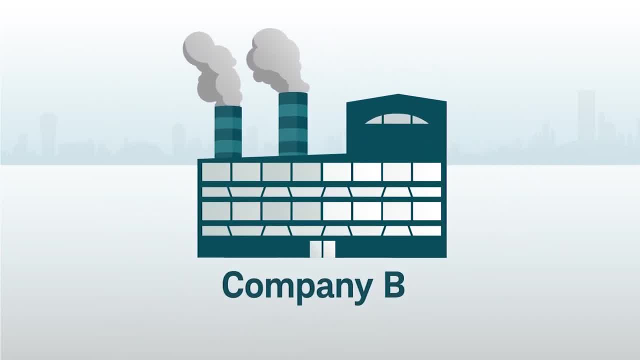 indicator that should be used when evaluating a stock. For instance, some stocks may have low P-E ratios because they have limited growth potential. If Company B only sells snow shovels in a state where there isn't much snow, then it isn't as likely to grow. However, if both companies